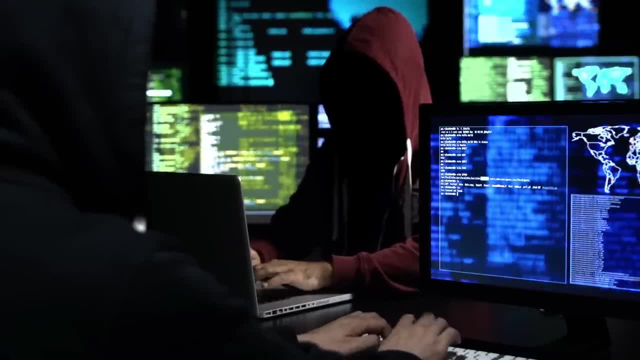 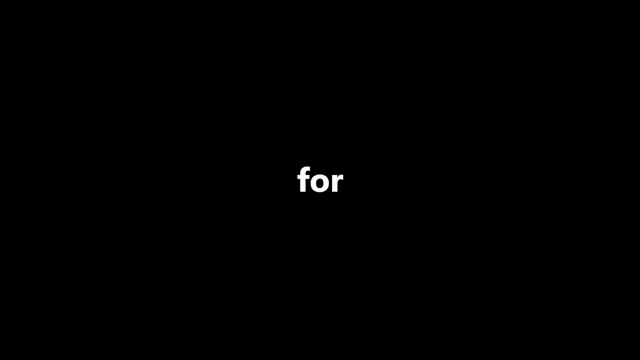 For years. that is how long a group of hackers were able to stay inside the Starwood Marriott network without being discovered. Oof How the heck does an unauthorized party stay hidden for this long? Well, in today's video topic, I will address popular methods hackers will use to stay. 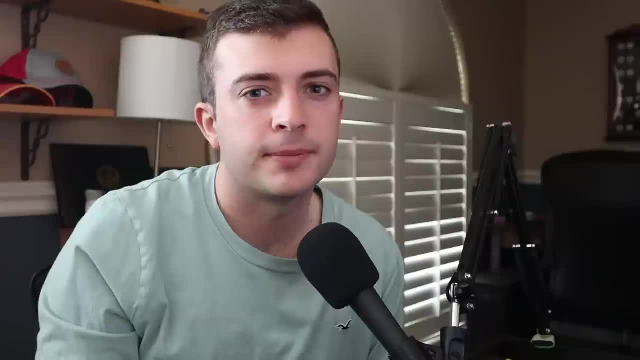 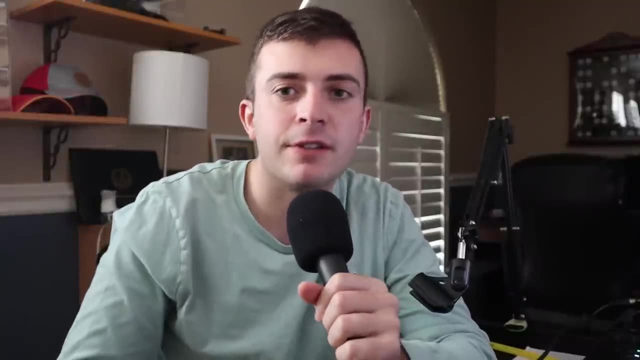 anonymous online while hiding their online footprint. So let's go ahead and get started. All right? No, the first step is not matrix level hacking, as much as we love it to be. It's actually physical security. Physical security is also referred to as operational. 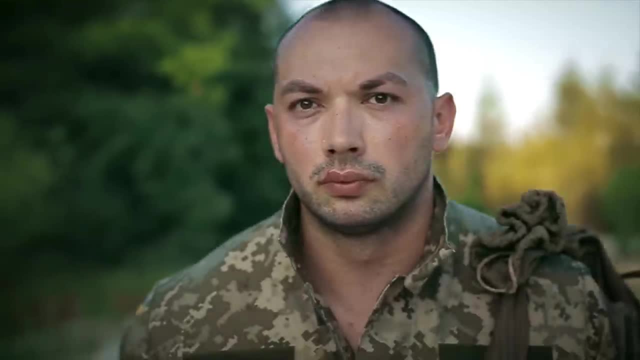 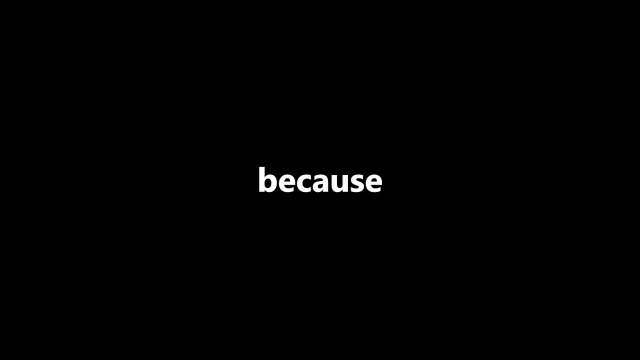 security or OPSEC. So if you're one of those you know military guys, you probably know about this. Or if you're just some random weird IT nerd, well yeah, you're probably gonna need to know about this too, Because guess how many times it takes to be successfully identified Once One. 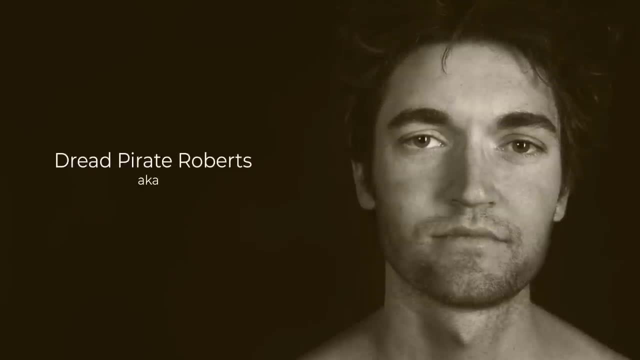 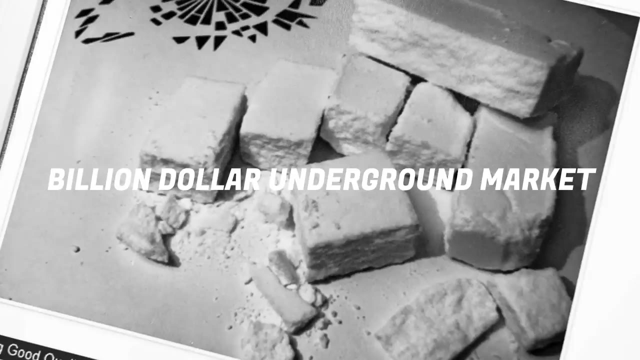 time, Like this guy right here, the infamous Dread Pirate Roberts or Ross Erbelich, or however you pronounce his last name, who founded the Silk Road, a billion dollar underground dark market place for drugs and other stuff. How did he get caught? Well, no, it wasn't through some extreme. 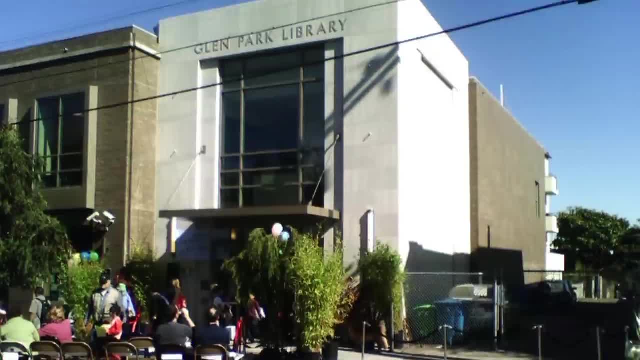 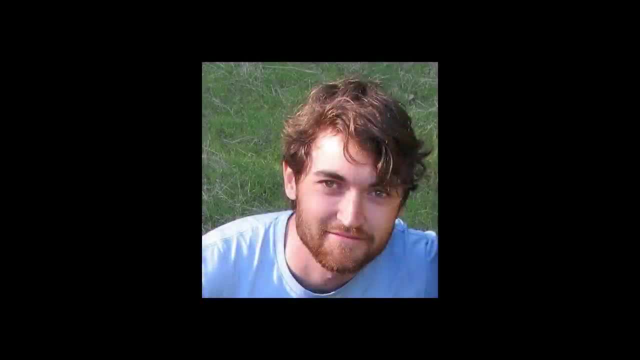 matrix level glitch hacking. It was his OPSEC. He got caught in San Francisco Public Library, his go-to place to conduct his fraudulent activity. And well, he did some bad things, such as often bragging about his work on his LinkedIn page using oblique verbiage, And he 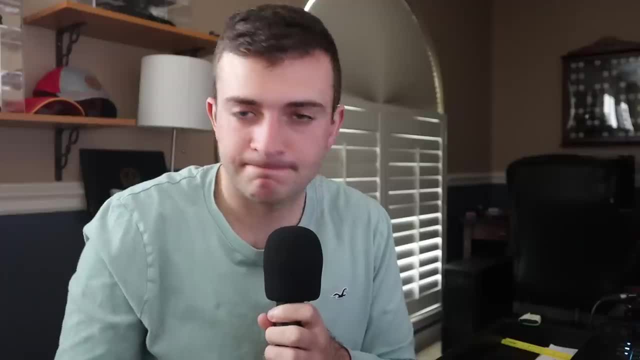 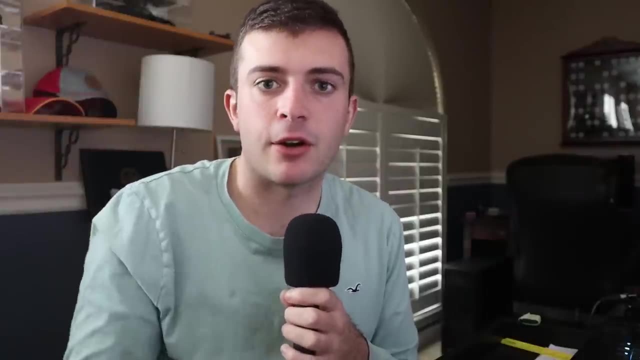 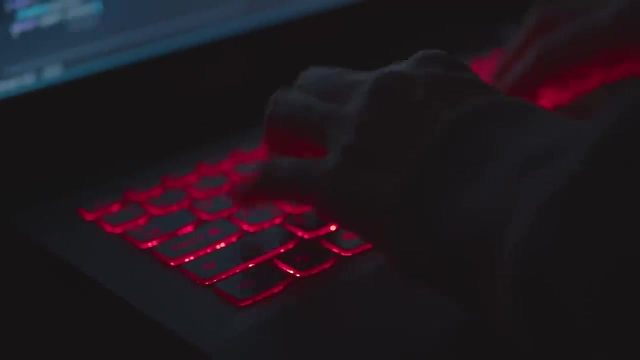 used his real photograph for his fake ID. So these are just a few of the critical elements which pieced together and led to his downfall, And these aren't technical in nature. It's habits and the public interactions that led to Ross's downfall. It is essential hackers be aware of their online and offline habits. 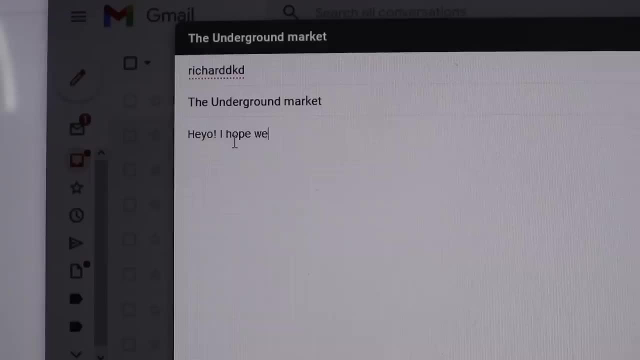 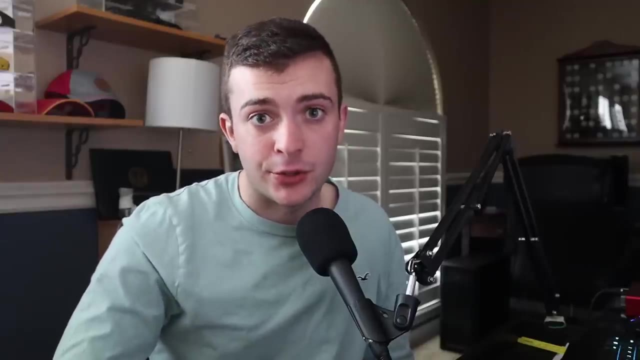 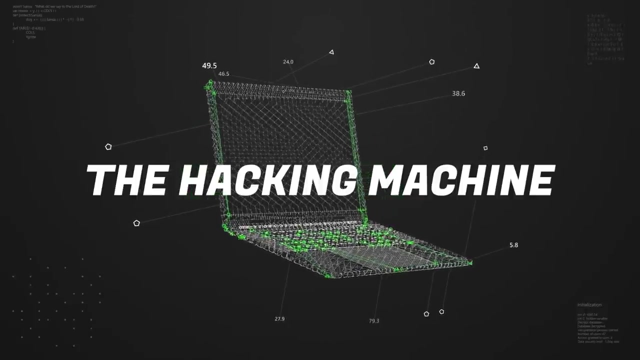 including where they use and connect their computers, their writing style, their social media posts and their social interactions in general. Basically, someone who's the exact opposite of me here on YouTube. Okay, so an attacker has their basic physical security down. What's next? Acquiring the hacking machine used to conduct your 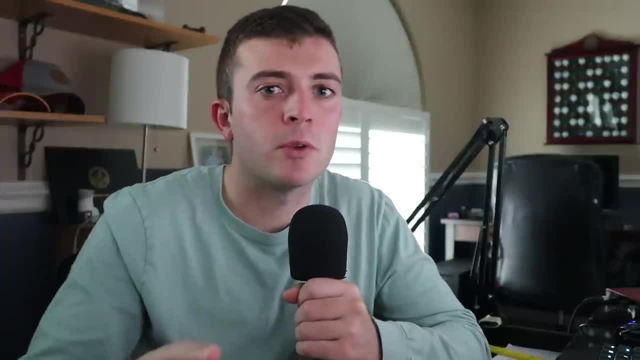 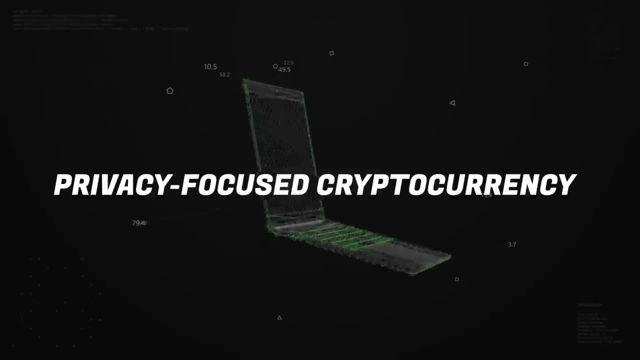 fraudulent offensive activities. First off, buy the machine with the most untraceable and mobile trail possible. Ideally, this is a laptop which is bought in a privacy-focused cryptocurrency form, such as Monero or Zcash. Once this machine has been acquired completely, wipe the operating. 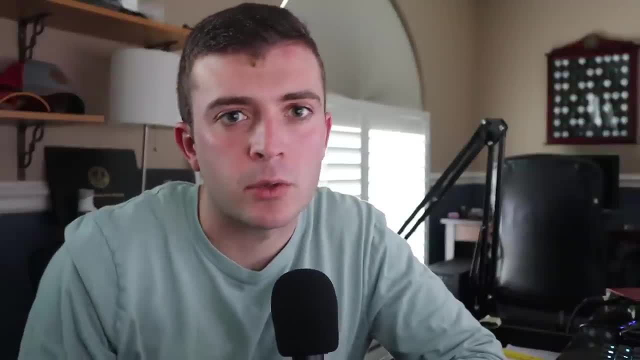 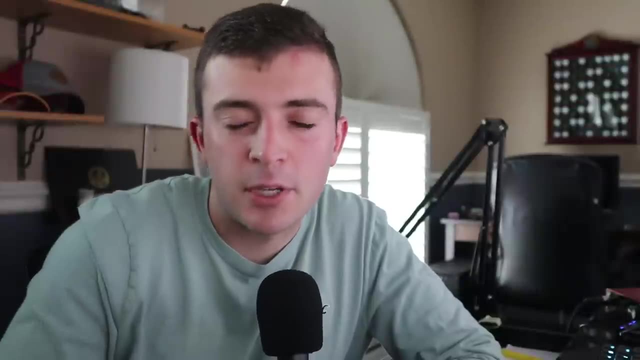 system windows no more- and immediately buy a USB stick to preload a live operating system. install This USB stick right here is a live OS, meaning there is no permanent storage, but you also have the ability to install a live OS. So if you want to install a live OS, 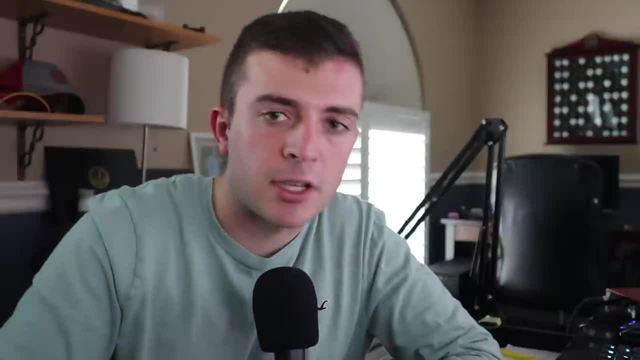 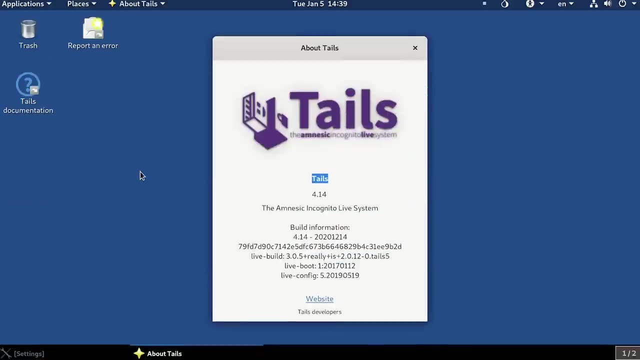 you also want to make sure to enable full disk encryption, just in case of full compromise. Now, when you're installing a live OS, it is important that you keep an OS distribution such as Linux Tails and Mine. Linux Tails is a suite of privacy-focused features and functionality. 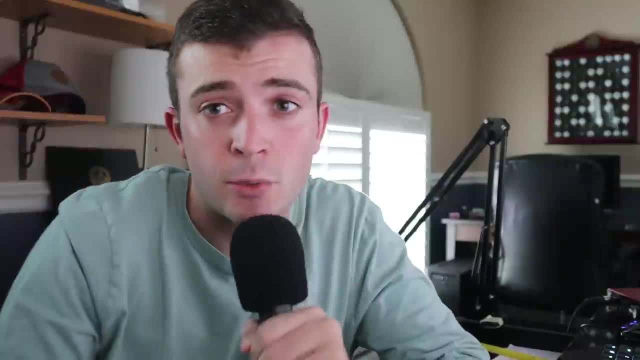 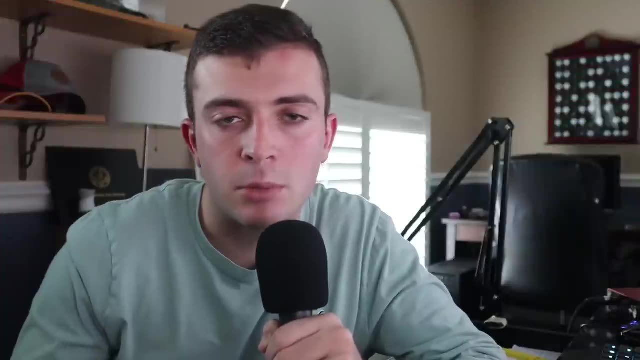 which allow an adversary to stay anonymous. All right. so what's the next step? you must say That is to go ahead and anonymize your identity and network connection. There are several steps to accomplish this. Now, any type of unique or pseudo-unique identity can be used to anonymize. 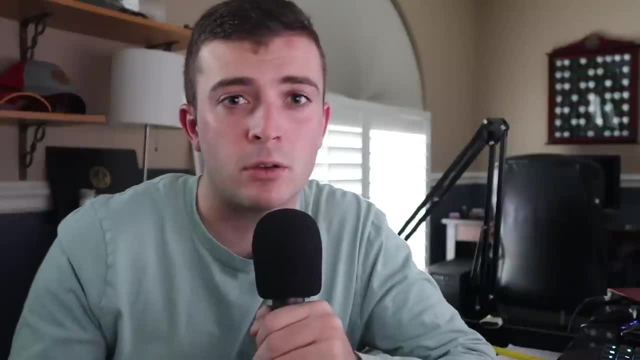 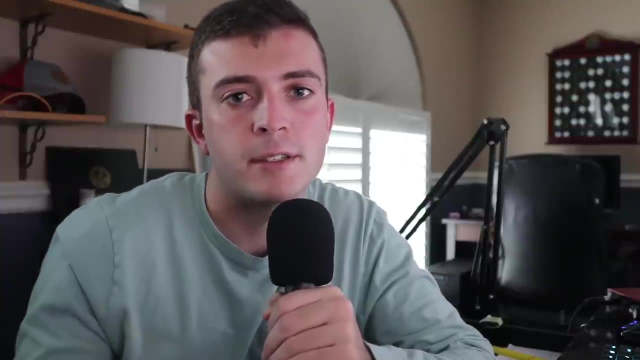 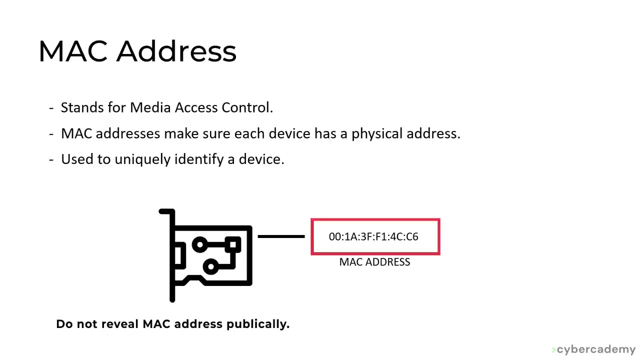 your identity and network connection. For example, if you have a mobile device, you may want to identify your device by using a MAC address. A MAC address is a serial number issued by the device manufacturers. It is used to identify a device on a local network and can be used to help identify. 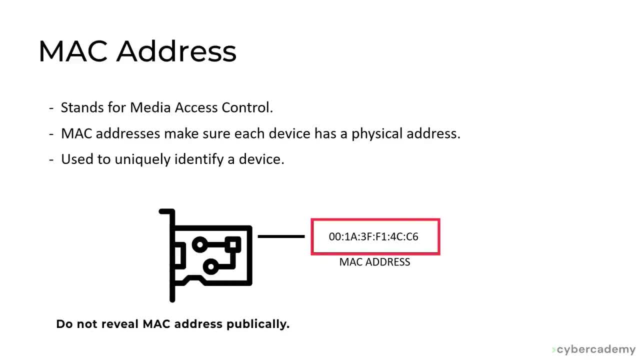 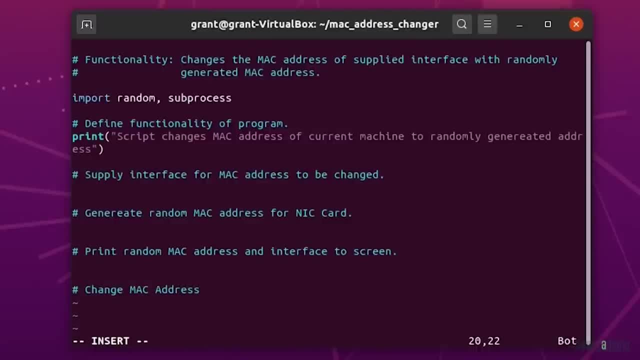 the geographical location of a machine. in some cases, MAC address spoofing or MAC address anonymization uses different MAC addresses to anonymize your device. For example, if you have a mobile device, you can anonymize your identity. There are different ways you can accomplish this. 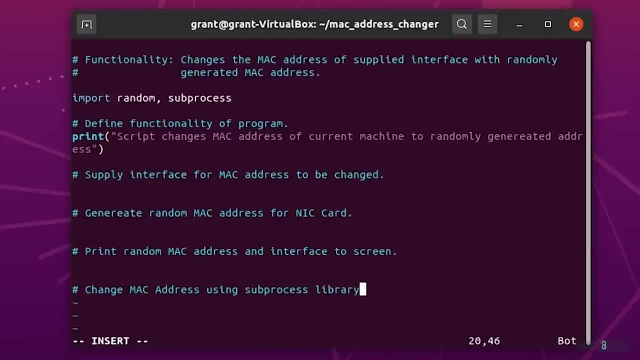 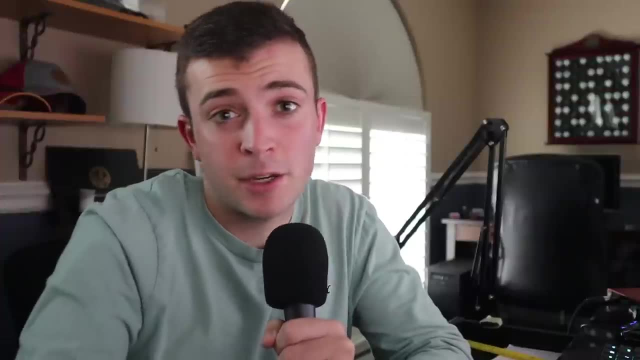 such as built-in programs, customized scripts and built-in tools. In Linux Tails, the MAC address is temporarily changed to a random value for each new session with Tails. Now, in addition to MAC address randomization, you're also going to want to anonymize the IP address. What is that? 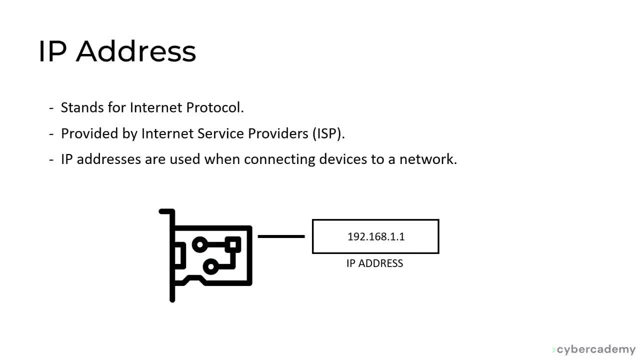 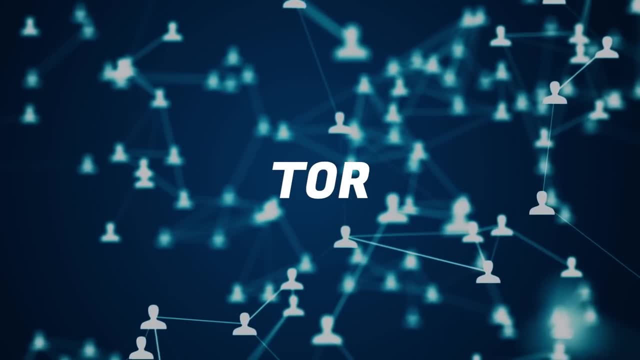 you must say An IP address is a network address assigned to all machines when connecting to other networks. To accomplish IP address anonymization, services such as VPNs, browsing and proxies can be used, but this is all with strict caution, Each of these methods. 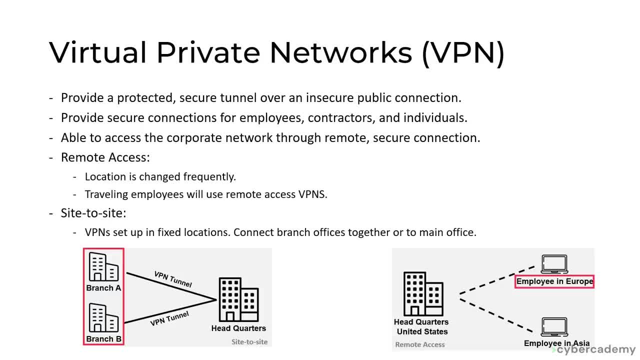 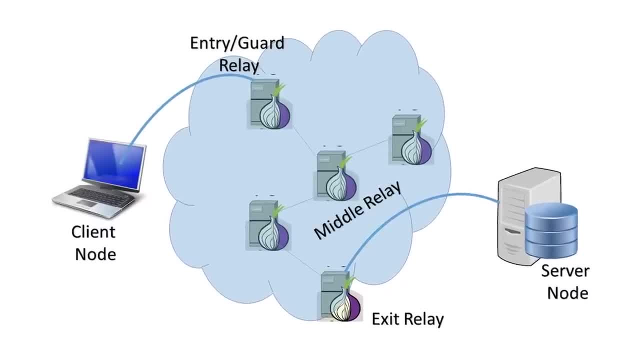 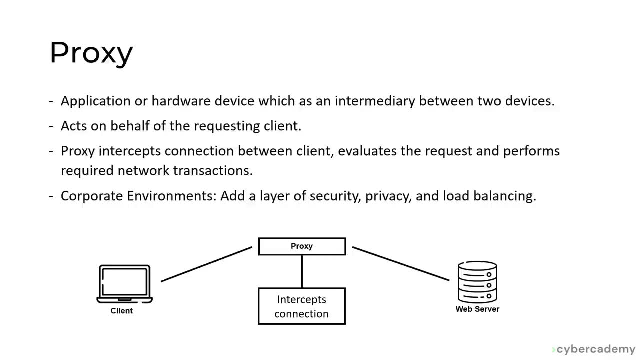 introduces intermediaries with assumptions of complete trust. VPNs extend a private encrypted network over a public network connection. Tor uses a network of computer nodes to balance a connection between different nodes across the world, and proxies can alter the location, appearing as if the originating request is coming from the proxy client. All three methods introduce: 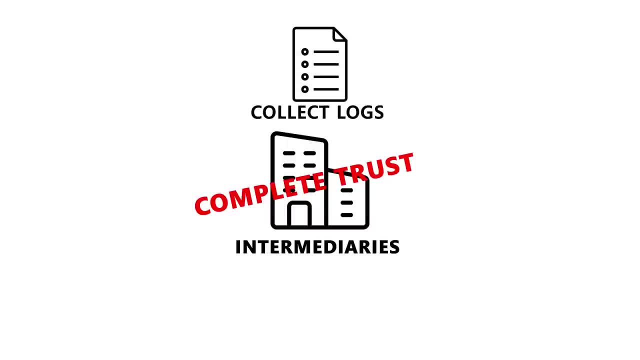 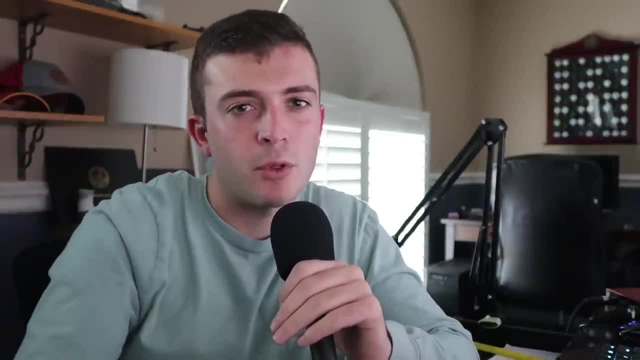 an intermediary or central location, which is a very common thing. in Linux, For example, if you log your traffic and send it to an authority in order to ensure 100% anonymity, you must never trust a central authority. But in a modern architecture such as the internet, that's. 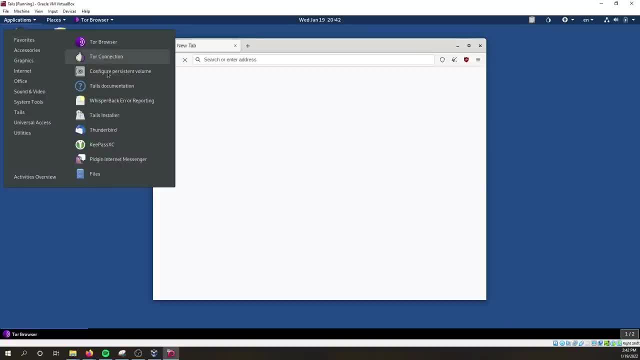 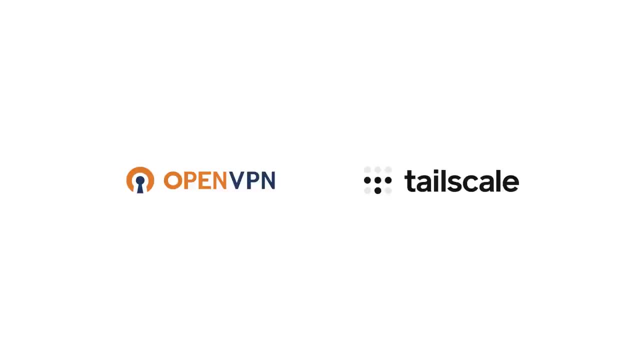 really not realistic Now to establish these types of anonymizing services. you could go ahead and use an open source project, For instance, for VPN servers you can use OpenVPN or Tailscale, and then you can install this on an attacker-owned or controlled device, or you could just use some. 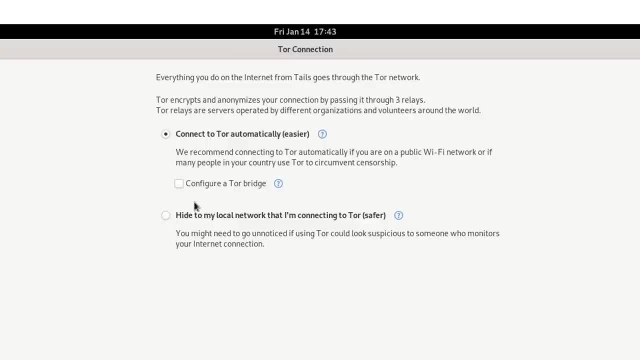 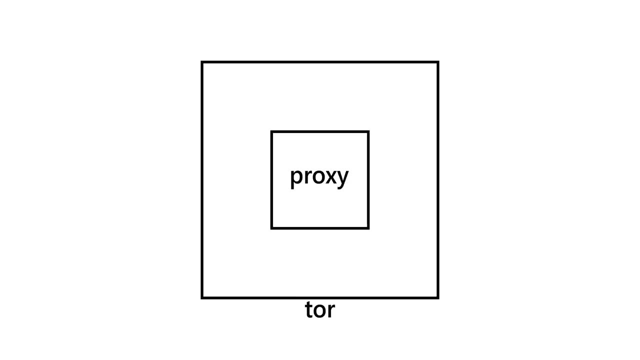 third-party provider For Tor. you can download and install a third-party provider and then you can follow the Tor project or use a distribution like Tails, which already has Tor routing enabled by default. A hacker can layer each anonymizing service upon each other, so a program like 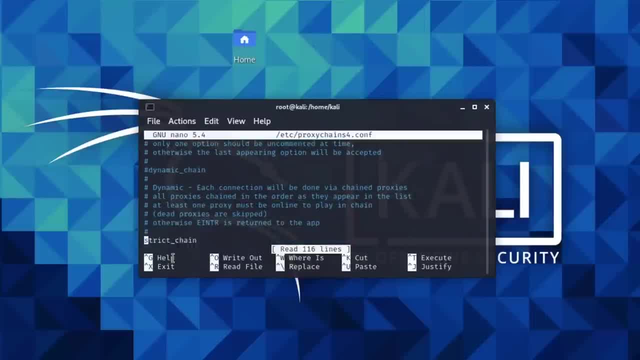 ProxyChains can be used to route internet traffic through a list of proxies on top of the Tor network. To set up this demo, I went ahead and edited the ProxyChains config file and set the chain to dynamic setting, which excludes all dead proxies. Then I also enabled DNS requests to be 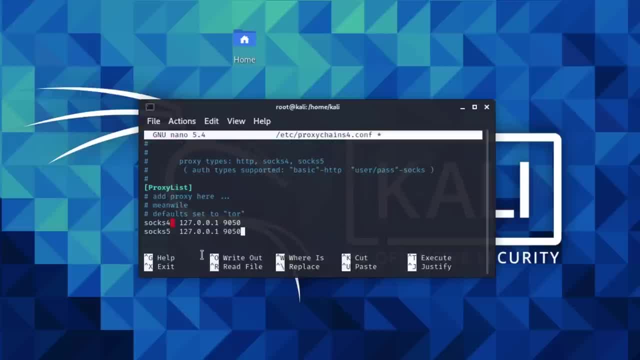 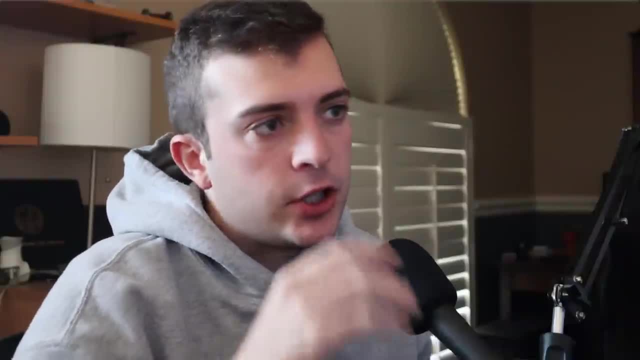 proxied through the network. To set up this demo, I went ahead and edited the proxy chains config file and I wrote down the default proxy server, which is the SOX5, through our loopback address. Let's proceed to go ahead and start up ProxyChains here. First thing we need to do is make sure that. 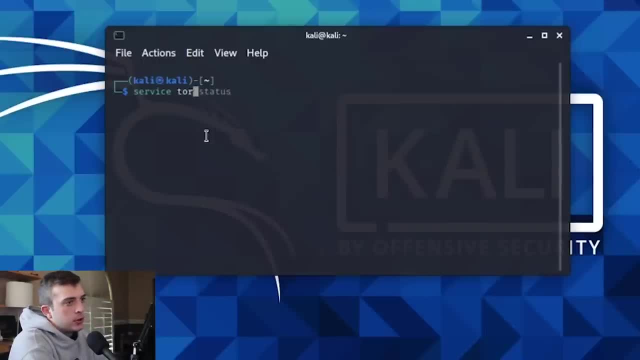 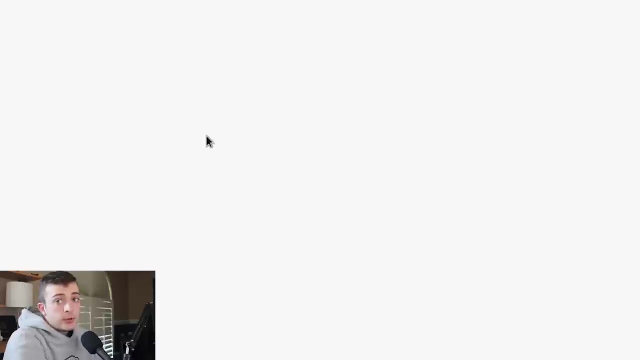 Tor is on, so we can go ahead and do a service: Tor start. Okay, once this is on, we can go ahead and go to our ProxyChains and we're going to go ahead and use duckgocom. Now, this will. 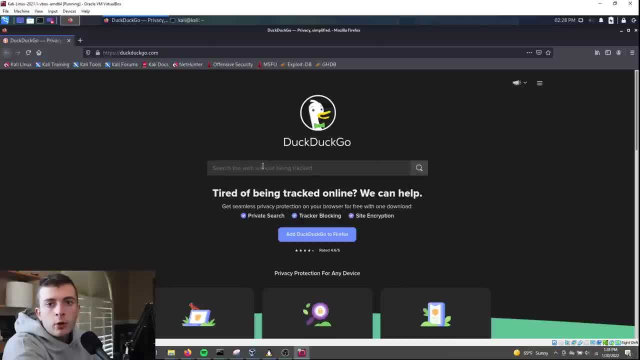 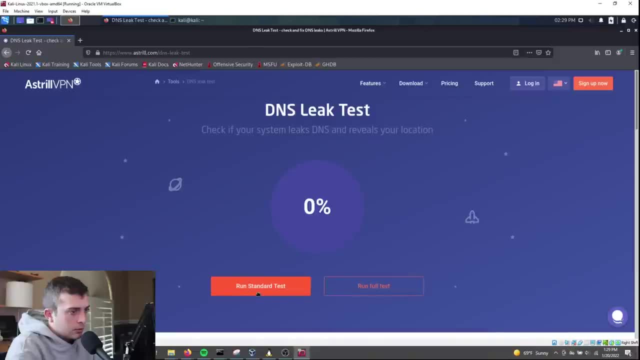 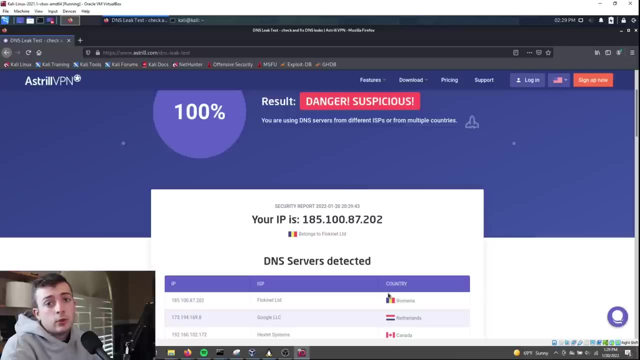 take a few minutes or it won't take anything at all, To see where we are coming from. we can use a DNS leak website, and I found this all through an article. so just go ahead and go to DNS leak And, as you can see, we are coming from Romania. so this is a basic way to layer both the Tor. 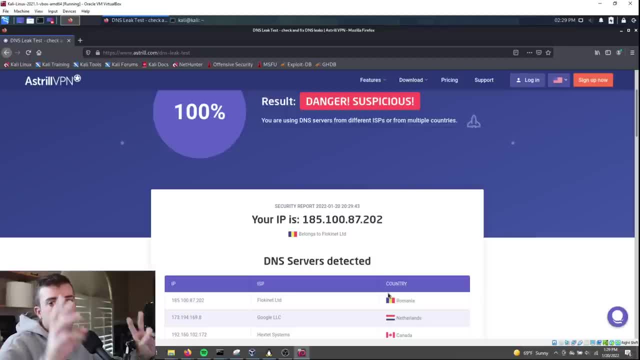 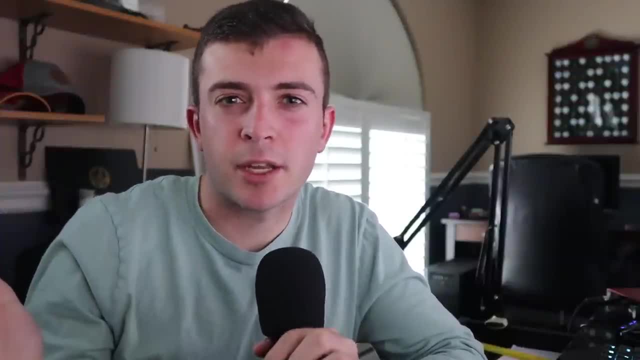 network and ProxyChains on top of each other to become anonymous. Okay, so after this step, it is finally time to ensure that you're not really working in the same environment, And that is separation of environments. You have to make sure that you're separating your. 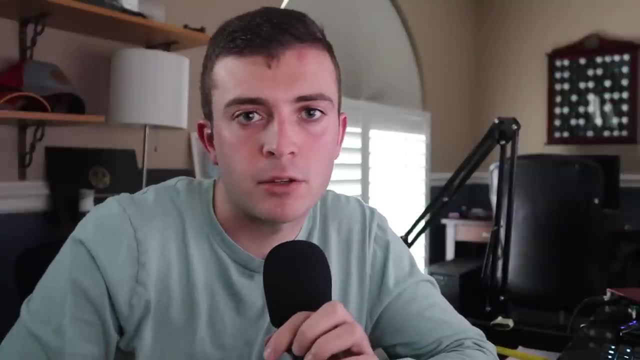 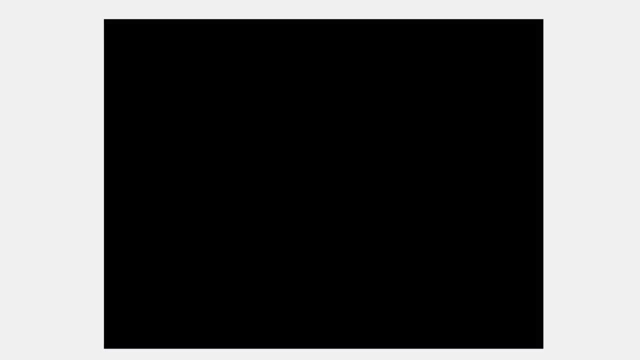 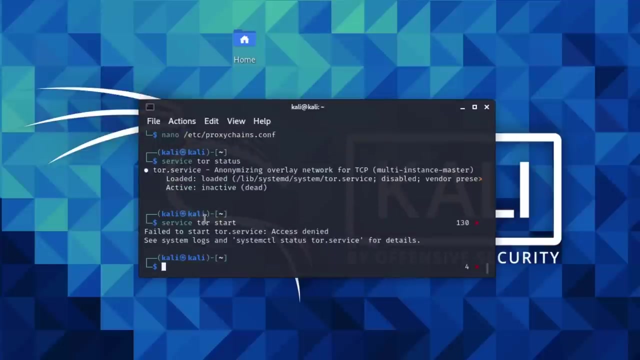 hacking environment from your normal everyday use environment. A classic example of machine separation is virtual machines and containerization. Use ephemeral or temporary environments when conducting offensive security activity. It is never a good idea to use one single environment for all activities. Computer machine isolation ensures evidence can be. 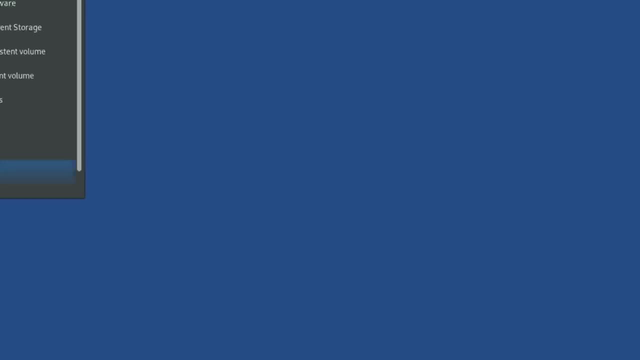 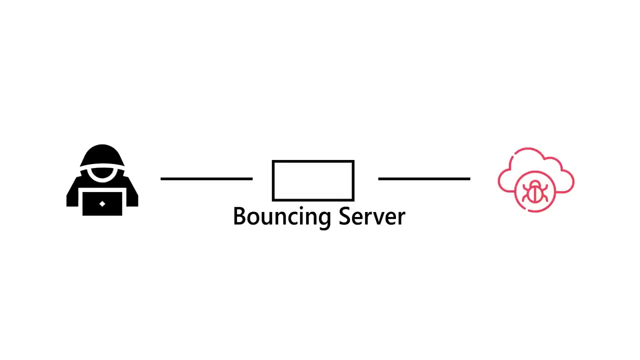 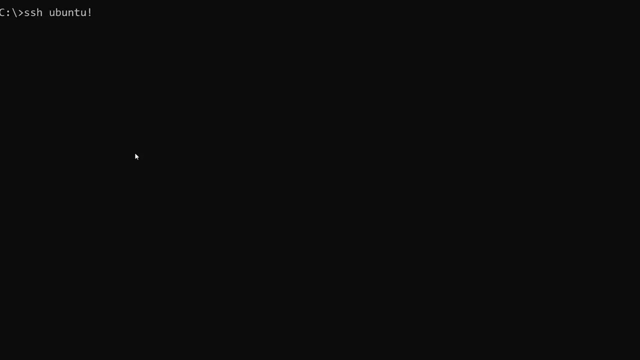 contained and then destroyed, and this can be really achieved through virtualization. Also, hackers can use a bouncing server to connect to their valuable infrastructure where their offensive tools and data lies. So some cloud party provider that doesn't really care about what happens on their machines. In this way, all a hacker has to do is have an SSH connection into. 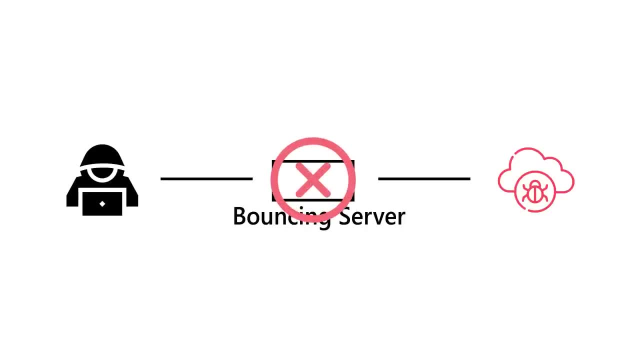 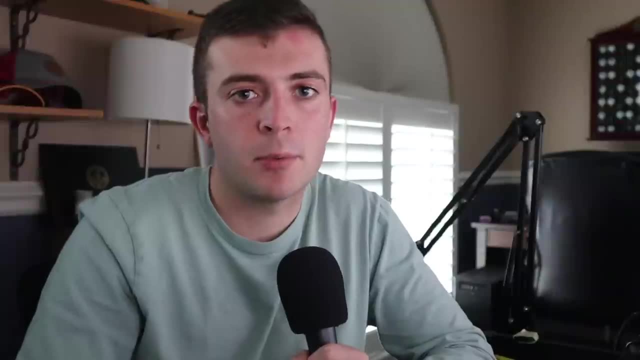 the server after they've anonymized their identity. Even if the bouncing server is destroyed or compromised, the hacker can curate and develop a new one within a matter of minutes. So, like I said before, you have to separate your offensive security work from your everyday work environment. 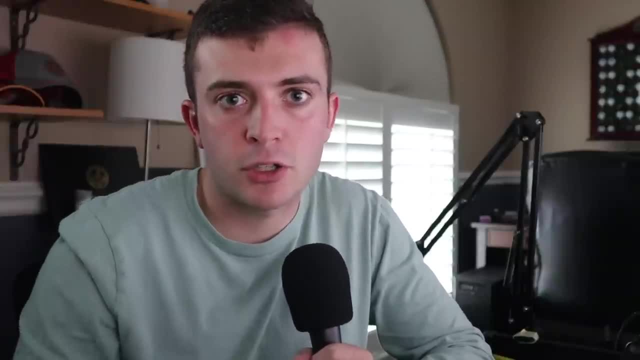 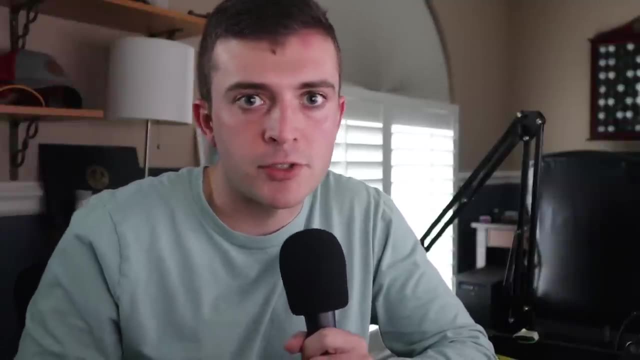 this case, it's important that you're also randomizing your network connection. So to do this, you can go into public Wi-Fi's and, you know, use Wi-Fi mapio, which is a resource to go, look for public, open Wi-Fi networks and make sure that you're randomizing exactly when you're you know. 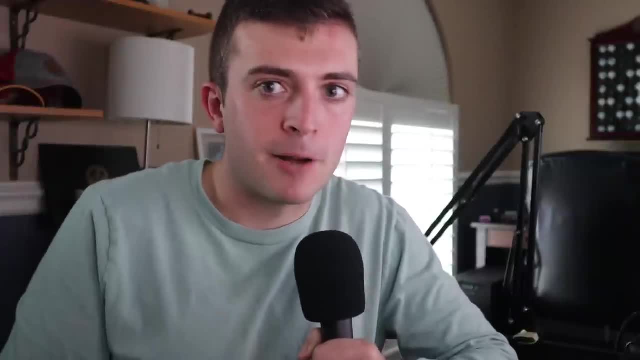 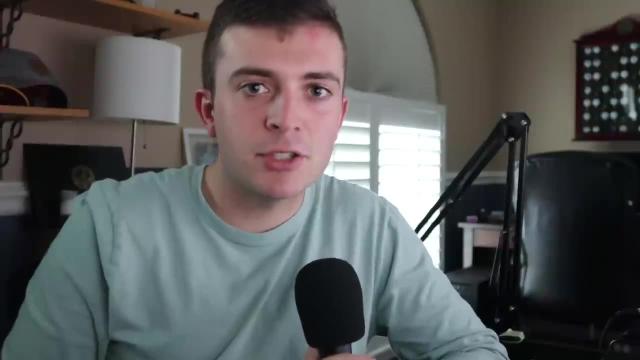 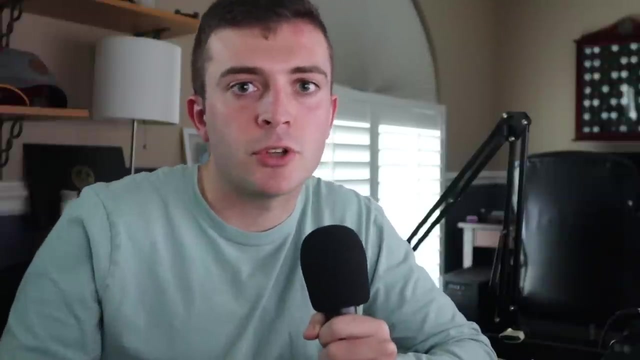 connecting to the Wi-Fi. Remember our good boy Ross. you know he well. you know what happened to him. Okay, so up until this point I've talked about anonymizing one owns identity, but I haven't talked about actual attack. So let's say a hacker has compromised a network similar to the Starwood. 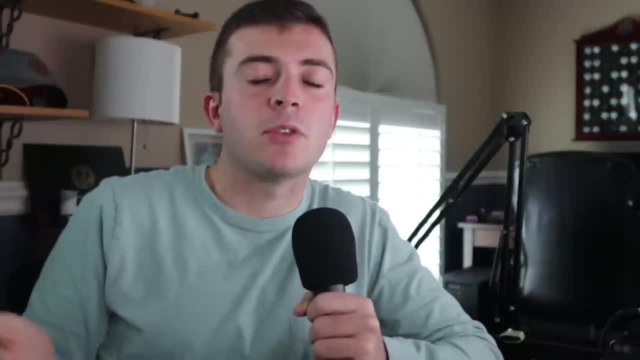 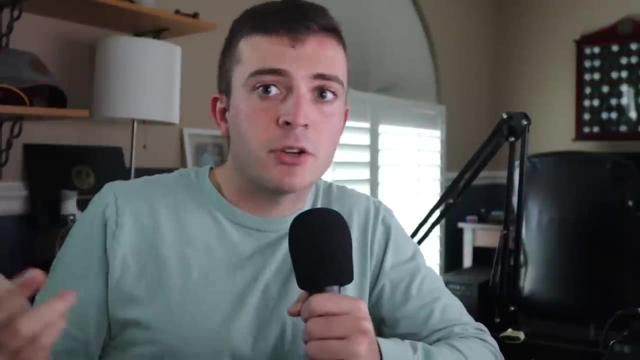 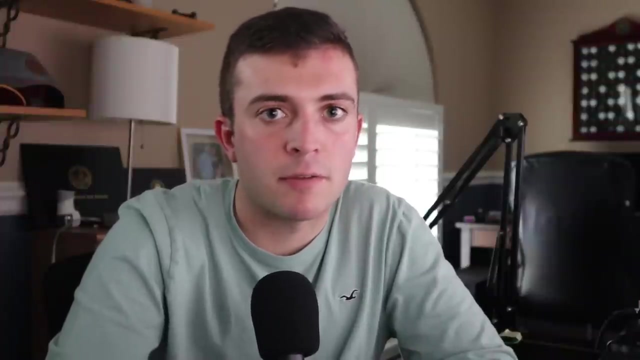 Marriott case. How can they go about? you know, covering up their online tracks within the network so they're not being detected by any security professionals like you and I. Once initial access has been established, it is imperative that attackers limit their offensive activity. So it's. 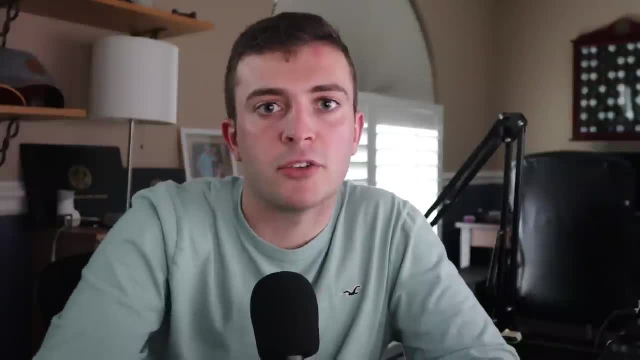 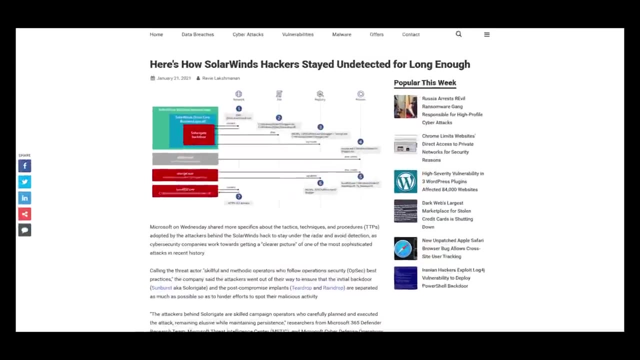 not a good idea to generate a whole bunch of lie and activity Once you're getting turned into the network. it's about stealthiness. Take a look at the SolarWinds attack of 2021.. The alleged adversaries kept the tracks hidden for months. 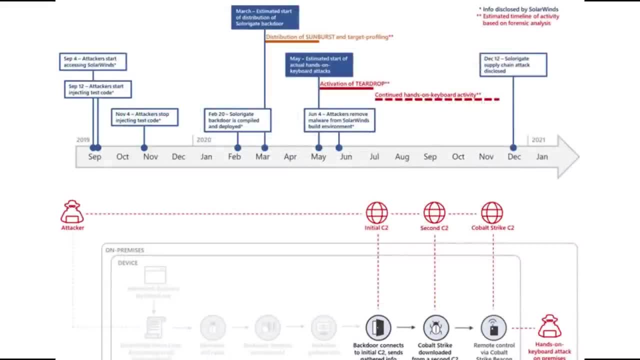 by slowly testing their capabilities through the course of those months. Initial access started September 4th of 2019.. And then by March of 2020 is when the distribution of Sunburst was deployed, And that took six months Now. in addition, a skilled adversary will analyze network and user. 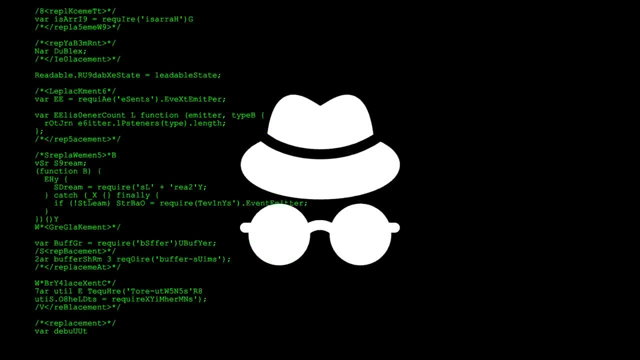 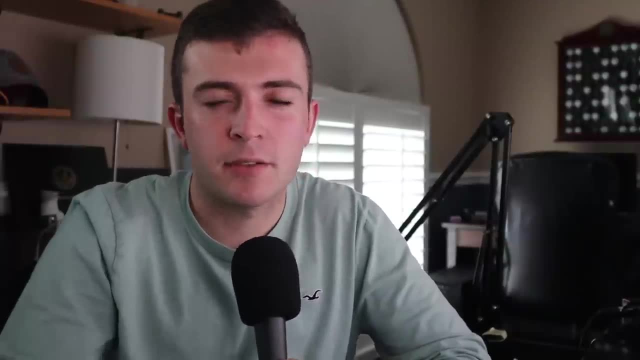 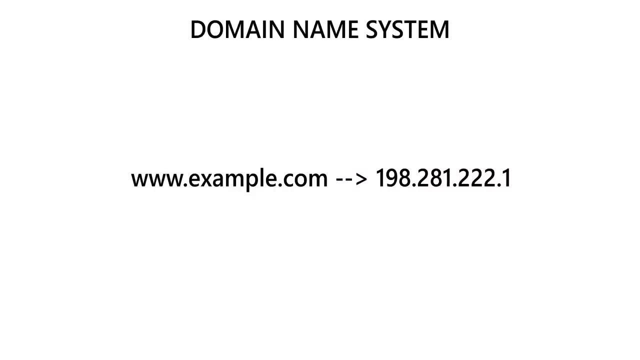 behavior and mimic this offensive activity as closely as possible, such as conducting their actions during the proper business hours. Next, hackers will blend their fraudulent activity with common network connections and protocols such as DNS tunneling. DNS, or the domain name system, is an essential component to a network translating. 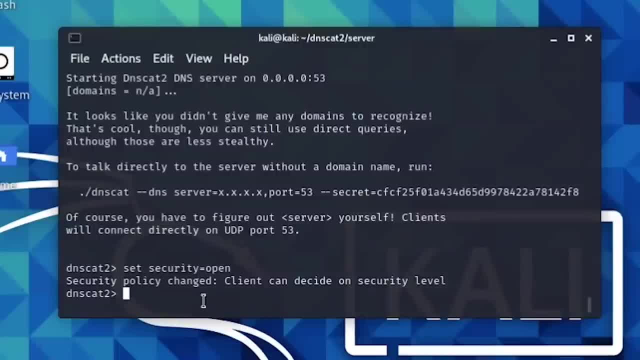 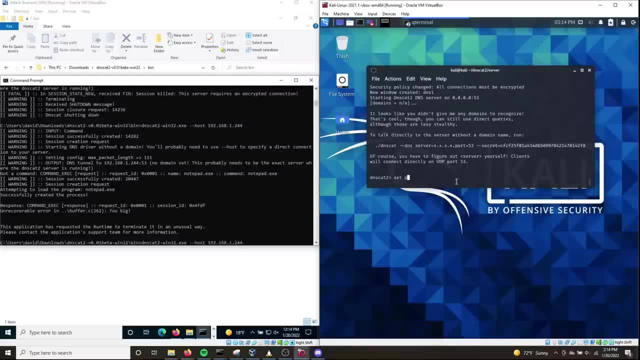 IP addresses into those web domains. Well, because DNS is essential, it's usually opened. So in DNS tunneling it uses seemingly harmless DNS queries to traverse between a private and public network. A hacker could use an encrypted connection and route their fraudulent activity through DNS. Take 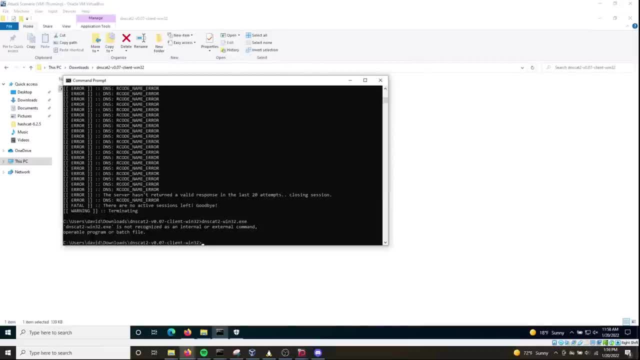 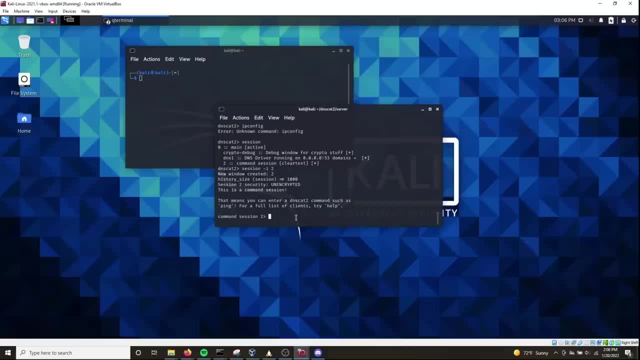 DNS cat to an open source command and control framework that lives out on GitHub, which is used to route traffic through DNS. In this demo I use the Windows machine to simulate a victim and a Kali machine to simulate an attacker. I downloaded DNS cat to utility on GitHub on. 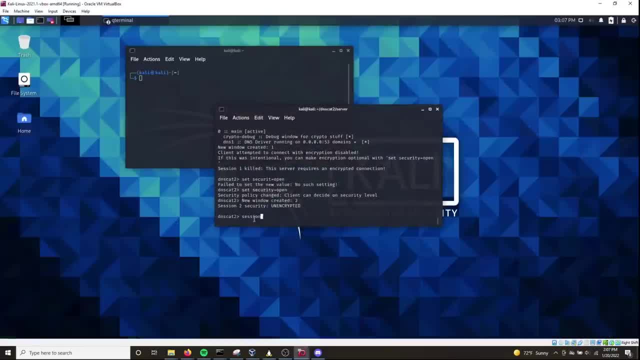 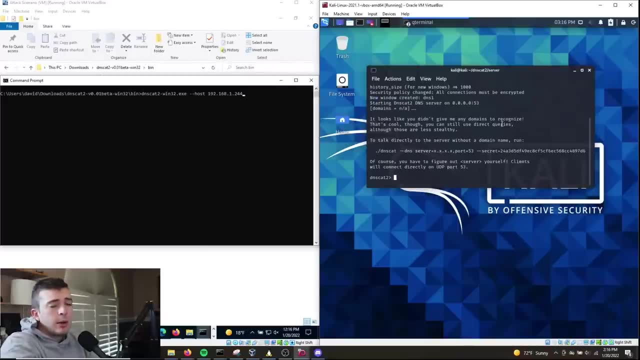 my Kali machine and then the victim payload on the Windows machine, which is an executable in this case. So if we go ahead and start the DNS cat to search, We need to set the security policy to unencrypted In a real world scenario. 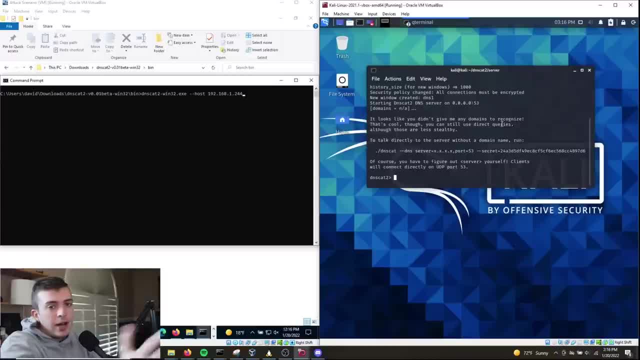 of course you wouldn't want to do this, but I'm a script kitty. So well, I'm just using this for testing purposes. and also, it worked. I'm a script kitty. Anyway, let's go ahead and get moving forward. So if we do sets, that will make sure that our security policy is to unencrypted Now. 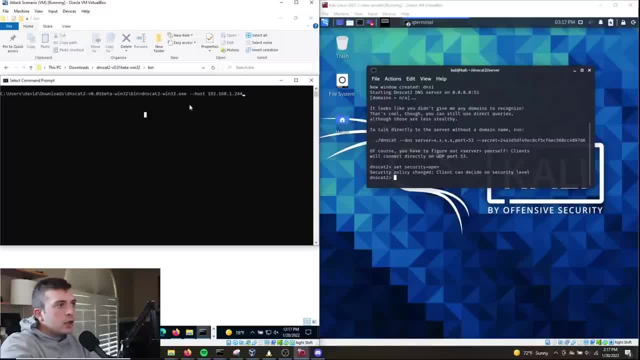 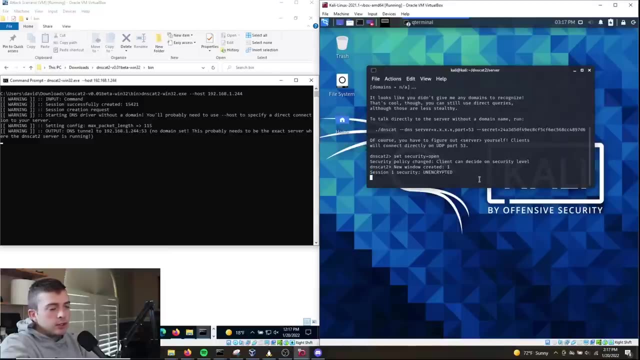 if we go into our Windows machine. I already downloaded the Windows 32 here, added the host, which is this machines. Let's go ahead and execute it And boom. as you can see, we now have a session and it's an unencrypted session. 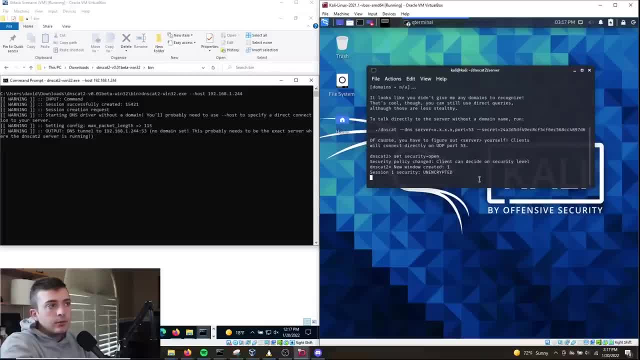 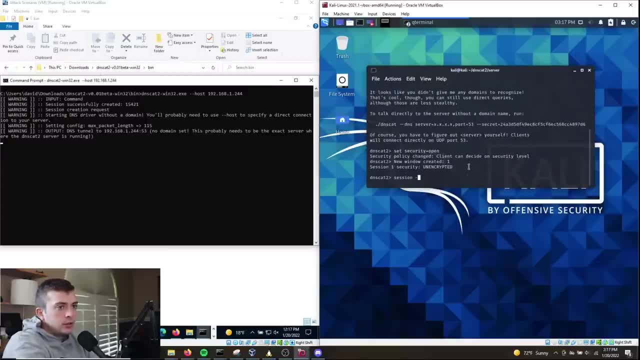 Now let's go ahead and see if I can get- well, I don't know- no pad plus plus or no pad open. So we, what we do here is we go into session I one and then we can see our list of commands. 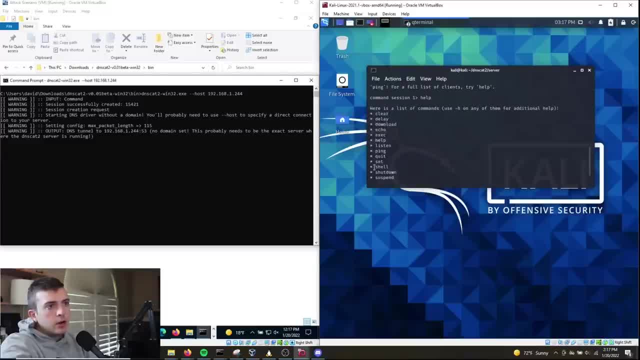 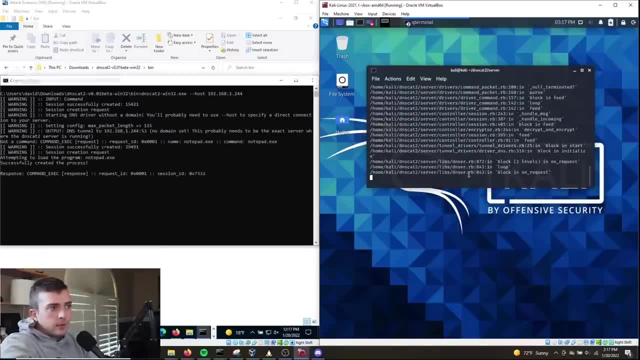 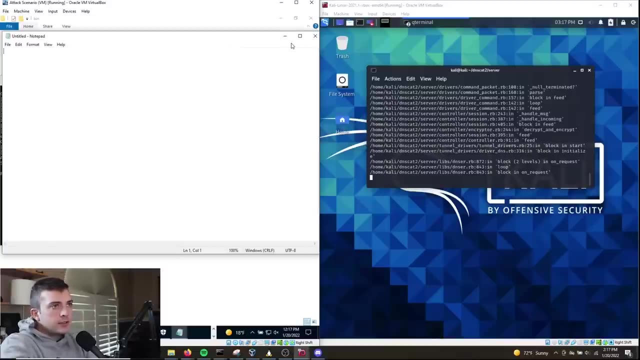 here that we can do So. for instance, we can ping or we can get a shell. but well, let's go ahead and do exec notepad And, as you can see, we now have a notepad opened and this is all tunneled through DNS.